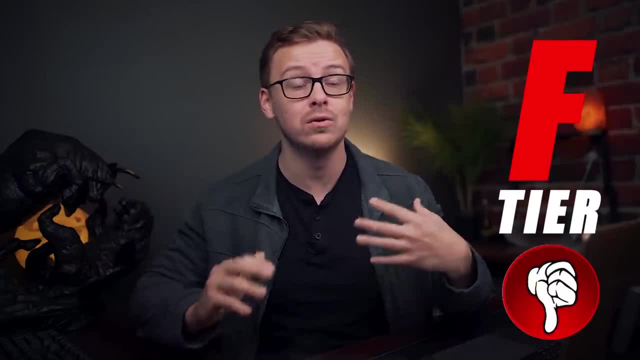 my choices. S tier is going to be the best. F tier is going to be the worst. I'm not going to explain it at all. You can watch all of my other videos if you want some explanation of why I'm doing this. So I'm going to try to cover all of the most common ones. 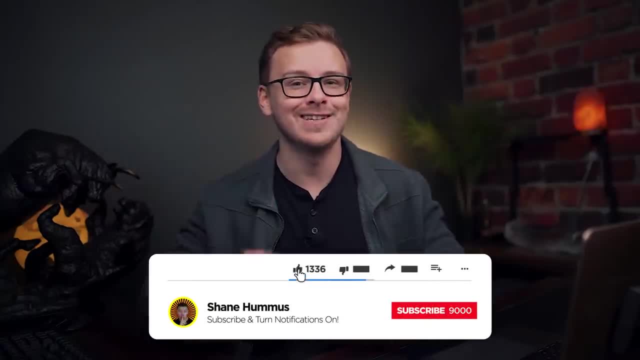 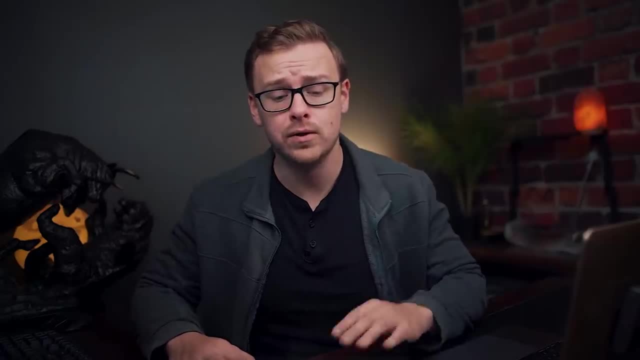 But let's jump right into it. right after you gently tap that like button, Hit the subscribe button and ring the notification bell. I'll wait for you, All right. first one on the list is going to be actuarial mathematics. Not sure why this was on top. I think that was a mistake, But this one's 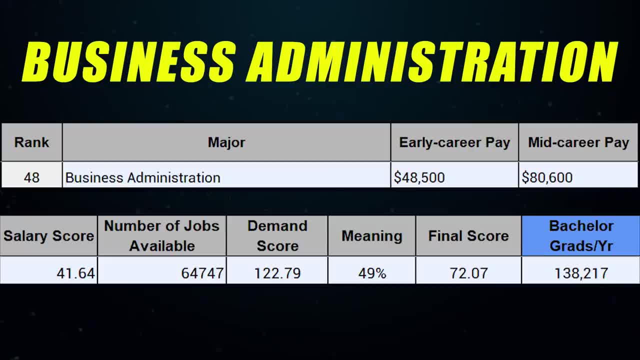 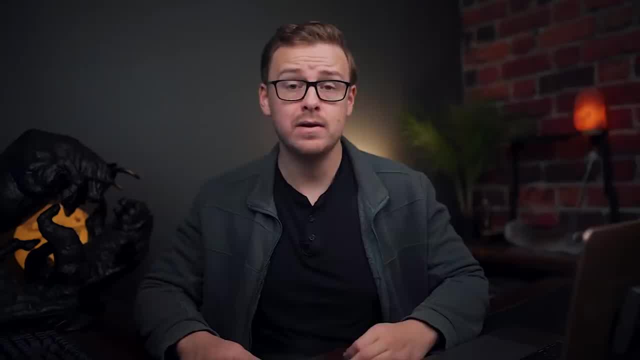 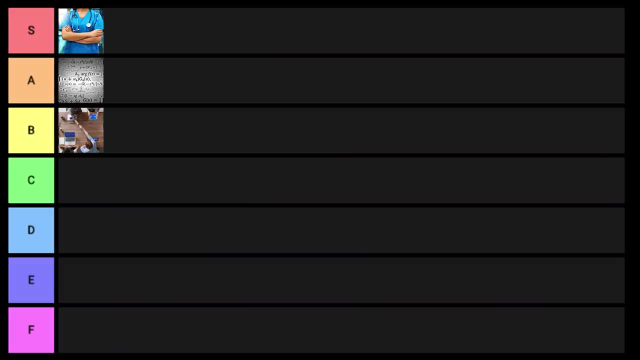 going into A tier. Next is going to be business administration, I think, for all different types of degrees. this one is going to go into B tier. Next one on the list is going to be nursing. So this would be a BSN nursing at the bachelor's level. This one is going into S tier. Next one on. 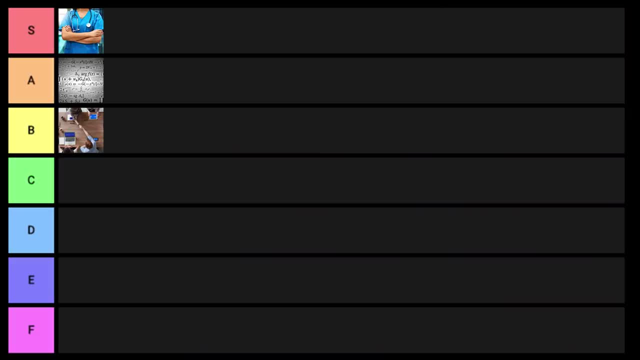 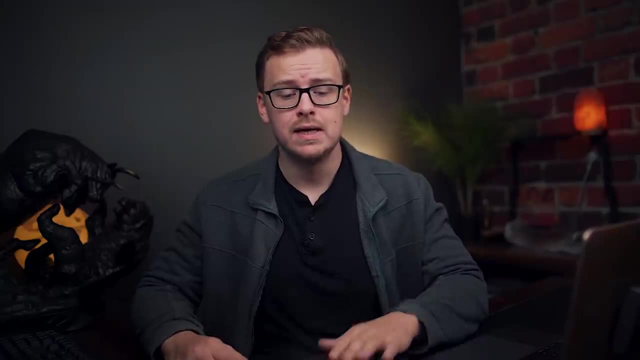 the list is going to be psychology at the bachelor's level. I'm going to go ahead and put this one into D tier. Next one on the list is going to be biology at the bachelor's level. I'm going to go ahead at the bachelor's level. I have to put this one into C tier. Next one on the list is going to 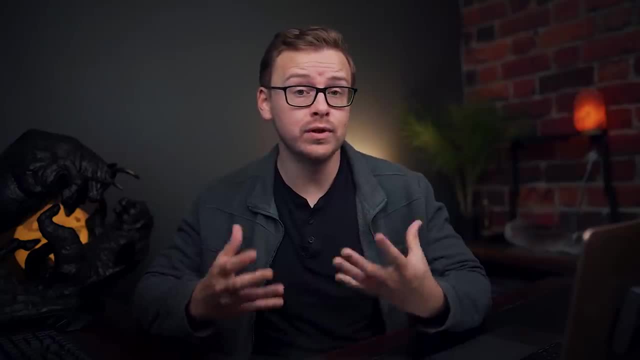 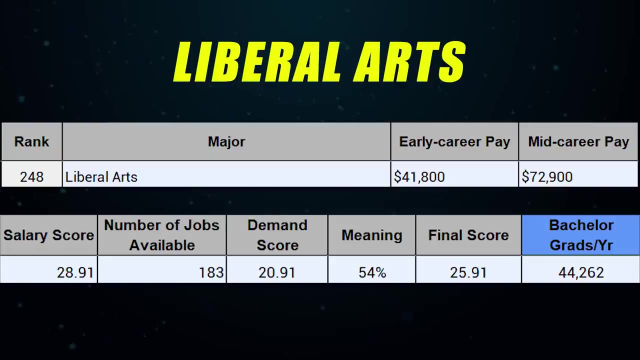 be accounting. This is a very common, really good degree. It's going to barely make it into S tier. Next one on the list is going to be liberal arts- very general degree. especially at the bachelor's level- super hard to find a job. This one goes into F tier. Next one is humanities. 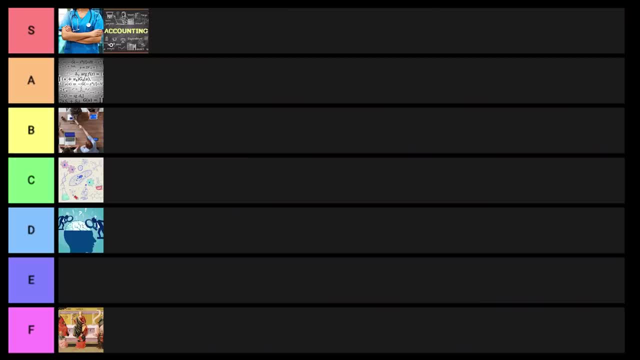 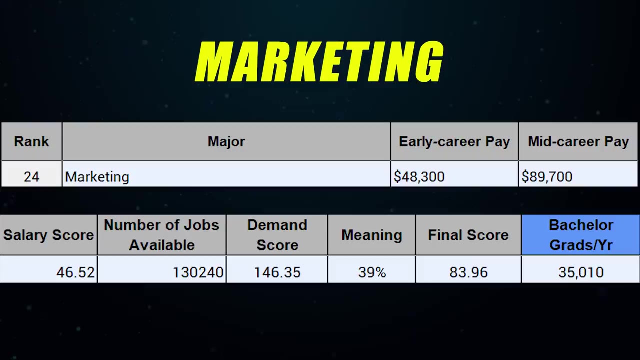 very similar to liberal arts too. general goes into F tier. Next one on the list is going to be a natural resources or natural resource management degree. This one's going into D tier. Next one on the list is finance. This one is also barely going to make it into S tier. Next is going to be 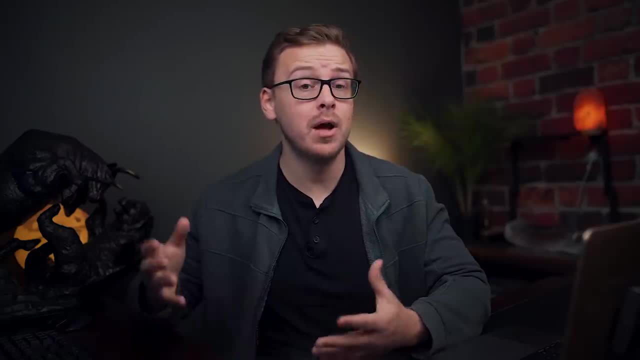 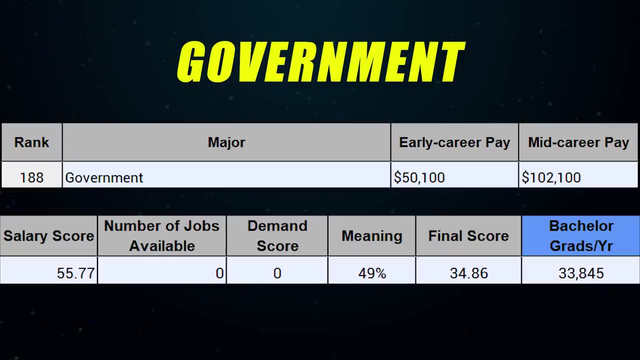 marketing. This one goes in A tier. Next we're going to talk about political science and this one is interesting. It's actually going to make it into B tier. Next is going to be government, kind of similar to political science. This one is going into C tier. Next on the list is going to be 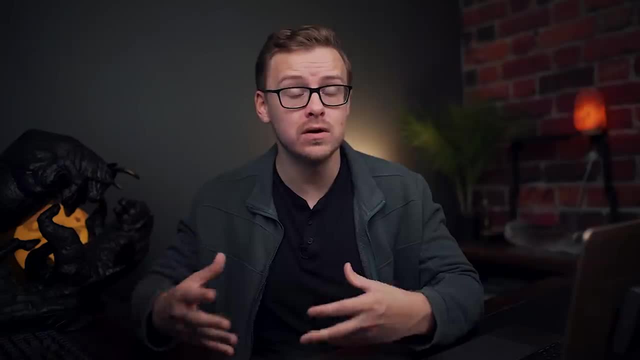 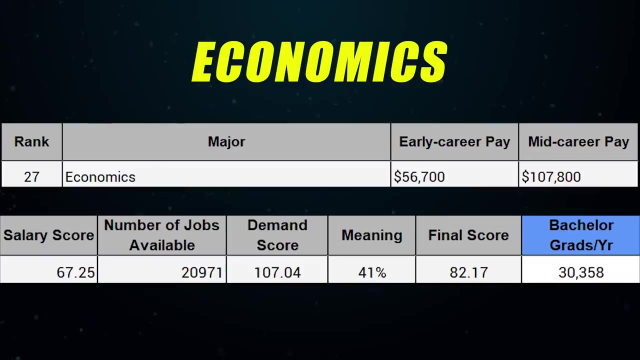 mechanical engineering. This one goes into S tier. It's an engineering degree but also very flexible. Next is going to be English language. This one is going to go into F tier. Next is economics. This one is going to be A tier. 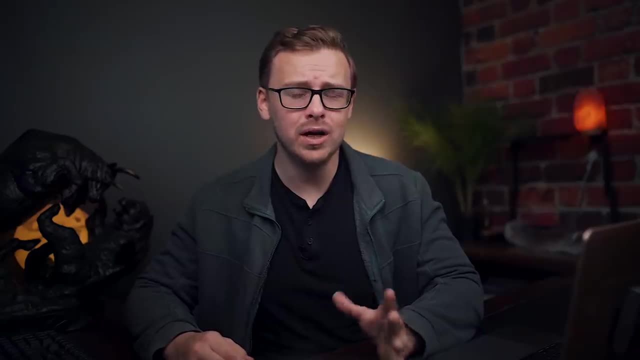 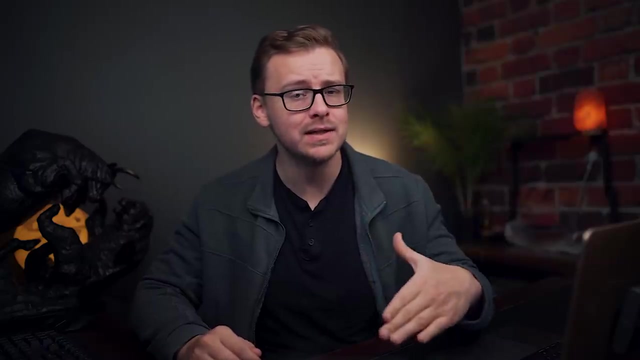 Next is going to be elementary education. I'm going to go ahead and put this one into C tier. I think it is kind of high C tier status. It's borderline, like B minus tier, like low B tier. Next is going to be: 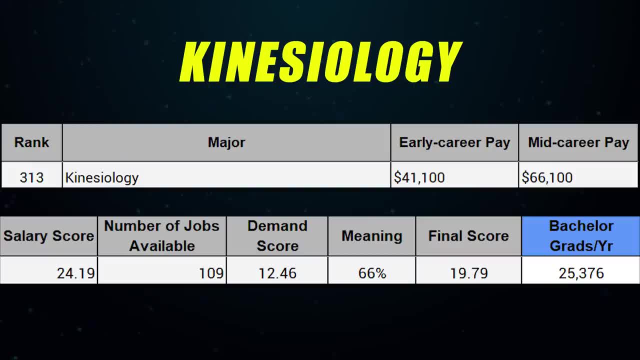 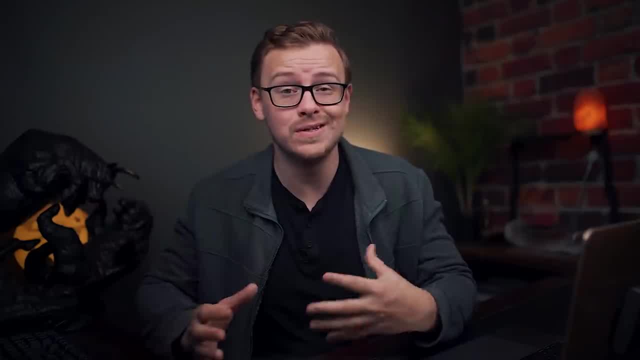 sociology. This one is going to go into D tier. Next is kinesiology. This one is also going to go into D tier. Next is exercise science. This one is one of the worst degrees, unfortunately. I think it's really interesting, but it goes into F tier. Next is liberal arts studies, or liberal studies. 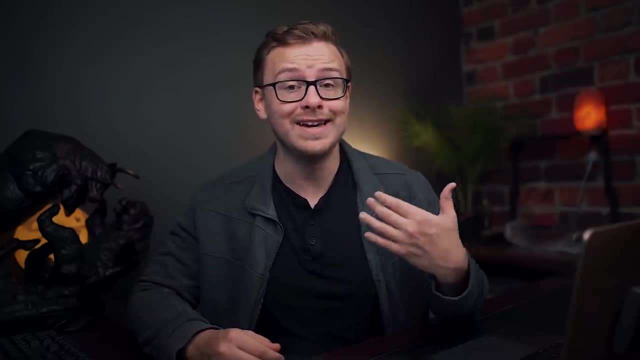 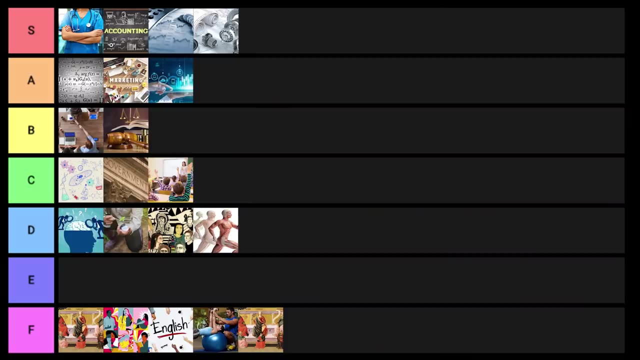 This one goes into F tier. Next one is going to be a history degree. Interestingly enough, it has somewhat decent statistics when you compare it to a lot of the other related ones. but I'm going to go ahead and put it into D tier. Next on the list is computer science. Of course this goes. 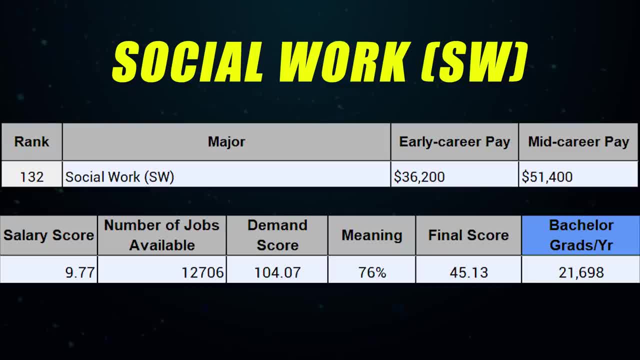 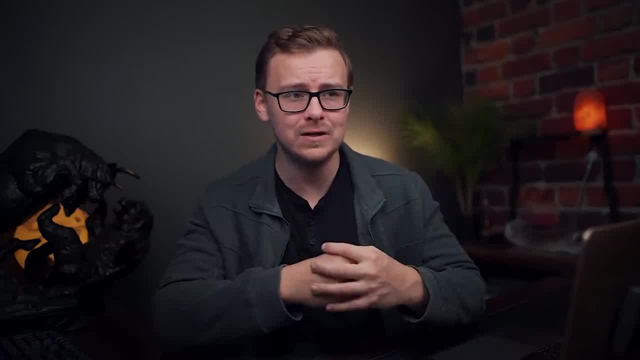 into S tier. Next one is going to be social work at the bachelor's level. This one, I'm going to have to put it maybe C tier. I almost want to put it high D tier status. It's almost in between. I'll go ahead and be nice and put it into C tier. 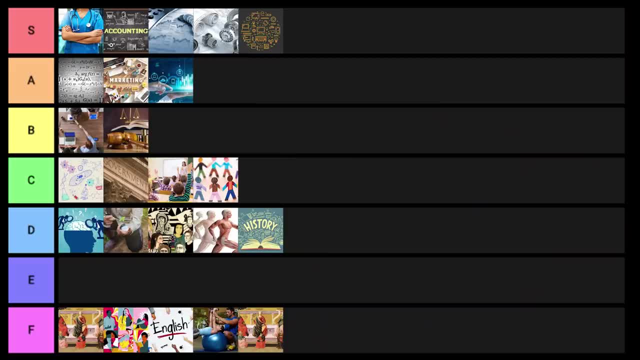 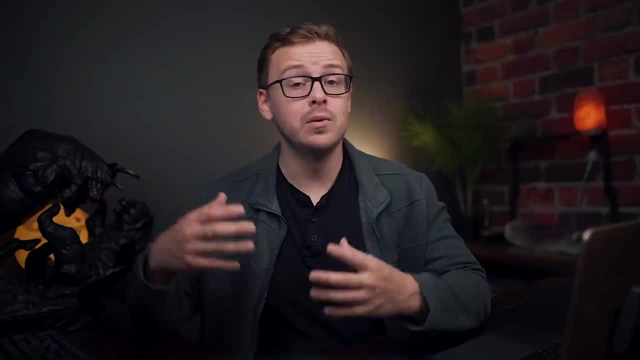 Next is going to be information science, A really interesting one. I'm going to go ahead and put it into A tier. Next is going to be mathematics. This one is also going into A tier. Next is going to be electrical engineering. This one goes into S tier Electronics engineering. very similar. This one is 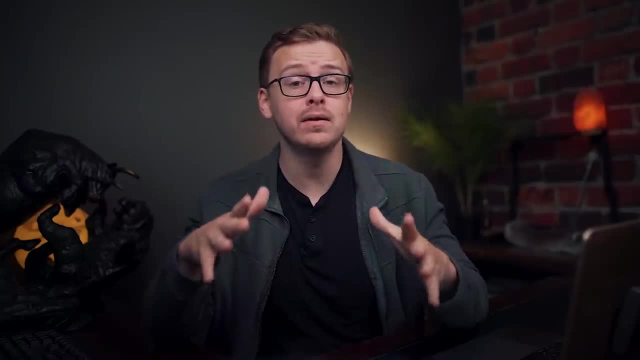 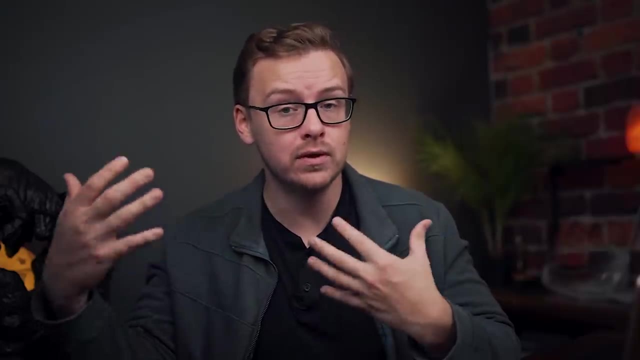 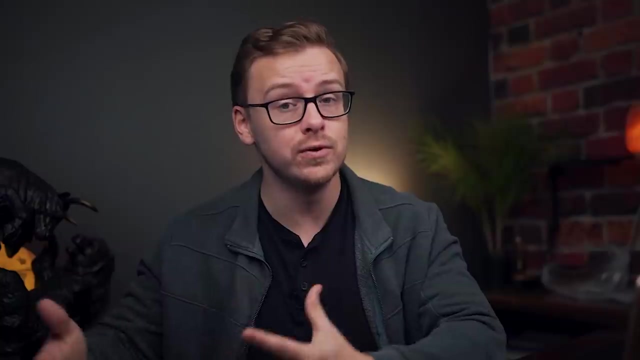 going to go into A tier And, by the way, in making this list, something that I changed from previous years, I assume that you are capable of doing the degree right, So I assume that it's something that you're going to be able to do because of the fact that you're interested in. You are going to be able to do it. 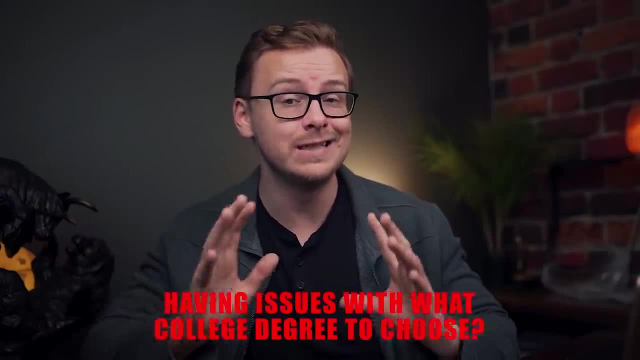 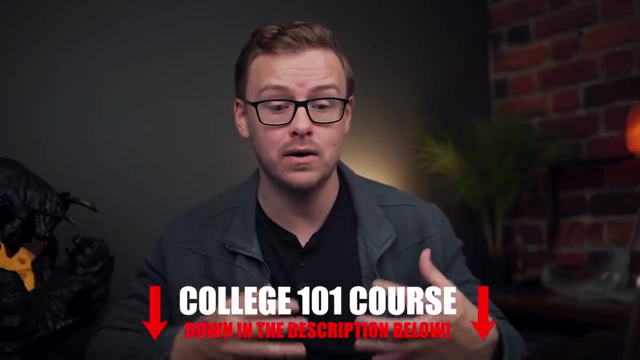 Engineering degrees are very difficult, So I decided to take the difficulty out of the score. In previous years I had that in there just because of the fact that there are a lot of people who go into engineering and then end up dropping out. So I'm 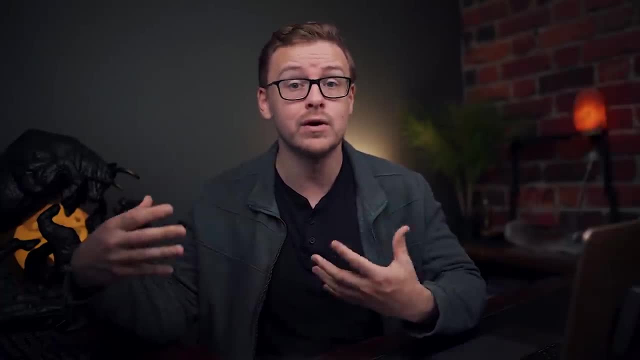 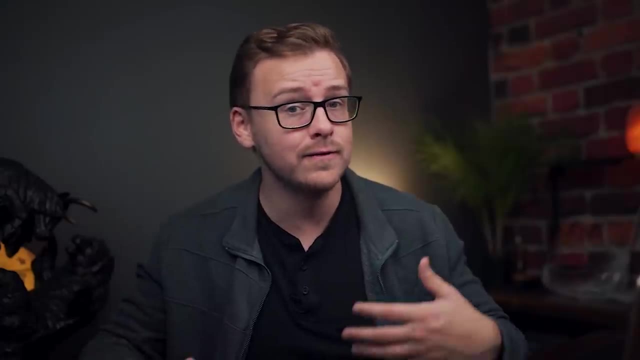 assuming that you are interested in it. You know, never do something you're not interested in, because it's going to be very difficult And if you're passionate about it you will be able to persevere. But if you're not passionate about it, if you're. 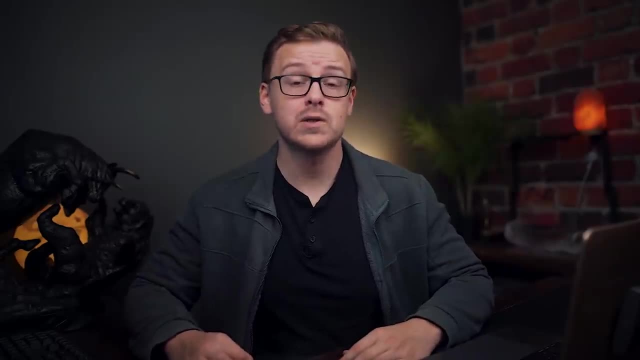 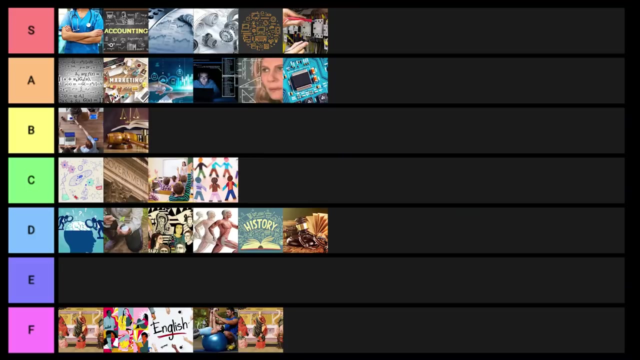 going to drop out just a little side note there, but I'm including that Next one on the list is going to be criminal justice. This one is going to go into D tier, Criminal justice administration. same sort of thing. D tier- Chemistry is going to be next on. 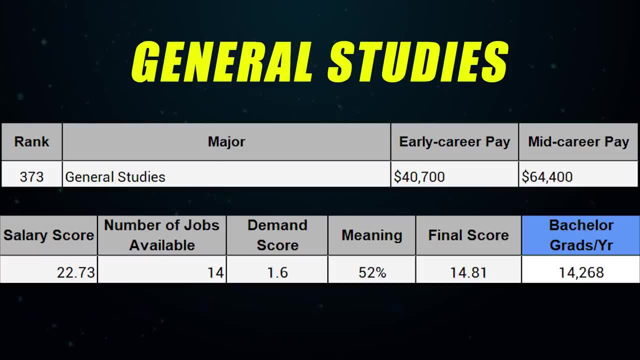 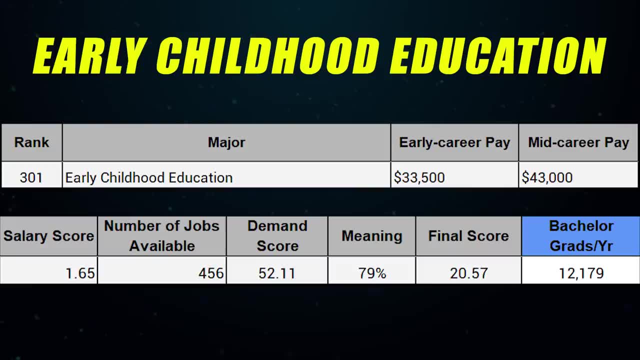 the list. This goes into B tier. General studies is next F tier for this. Civil engineering is going to be next on the list. I would put it in low S tier status. Early childhood education is next Another education degree. I'll put this one in C tier, Health. 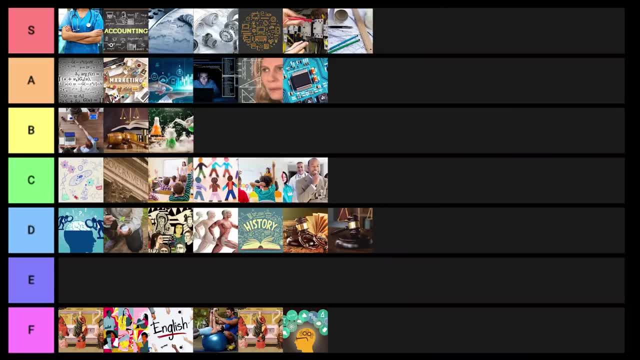 administration is next on the list. This one goes into high C tier status. Next is going to be journalism And this one is also going to go into C tier. Chemical engineering is next And this one goes into S tier- Art. history goes into F tier- Art goes into F tier- Communications goes into D tier- Mass. 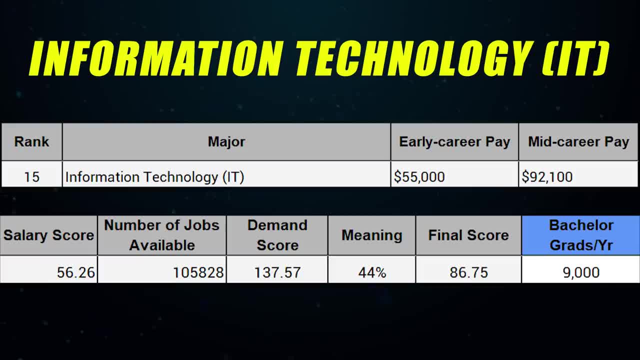 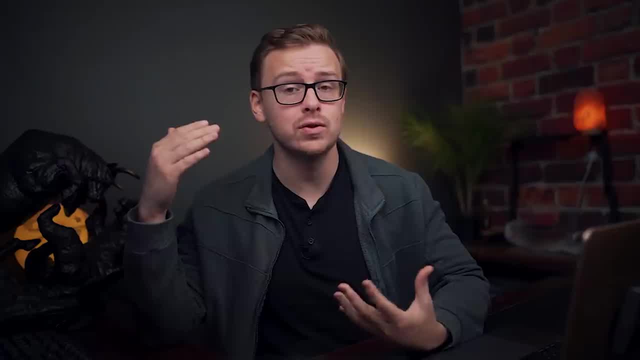 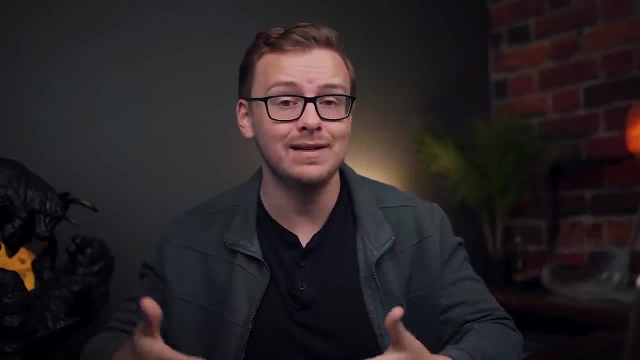 communications also goes into D tier. Information technology at the bachelor's level goes into S? tier. There's a little bit of controversy about that one, just because of the fact that you actually don't necessarily have to get a bachelor's. But when you look at the numbers, if you do get a bachelor's it's not going to be like a scam. Okay, so S tier, but with an asterisk. 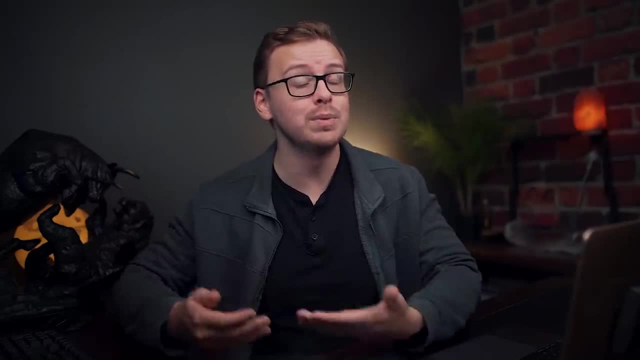 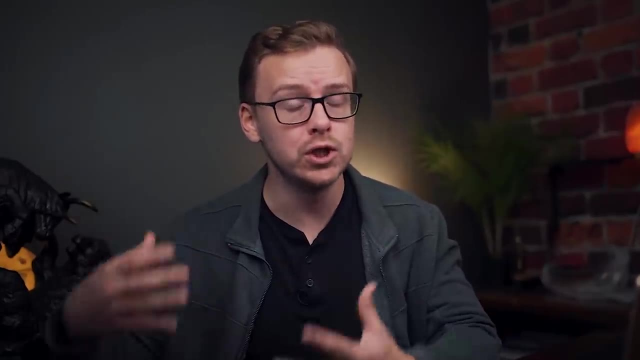 A lot of different technology related degrees are like that, where you could potentially teach yourself. or you could go another route, get some type of certification or go to a boot camp, But if you want to go more of a traditional educational route, that is also a good choice, as. 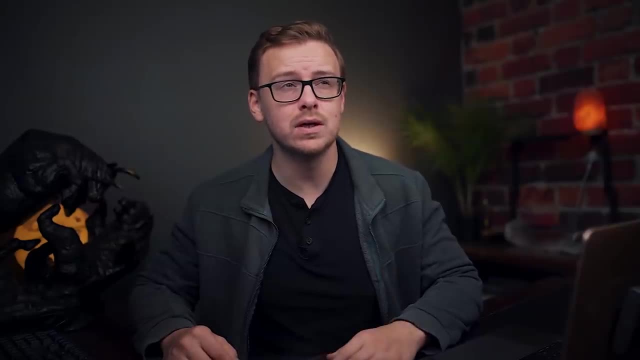 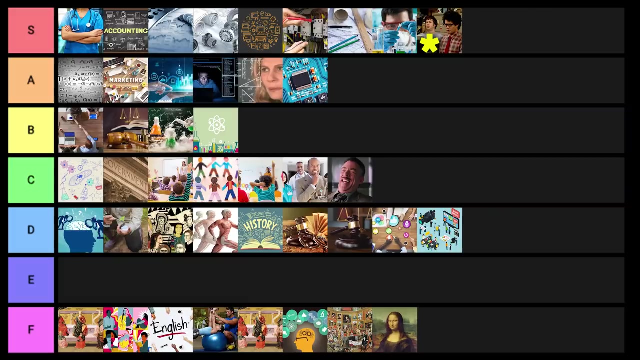 well. Next is biochemistry, And this one is going to go into B tier. I would say it's kind of high B tier, though. Next is family studies, And this one goes into F tier. Drama goes into F tier. Theater arts goes into F tier. International relations: this one's 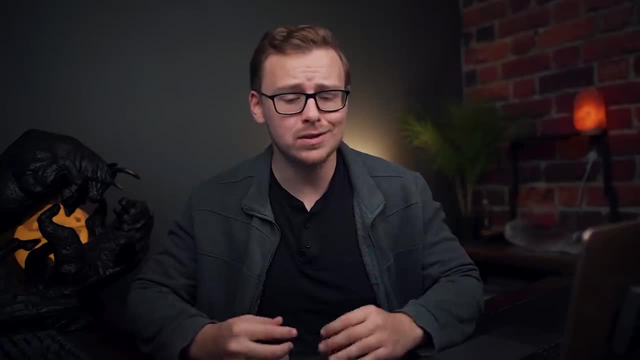 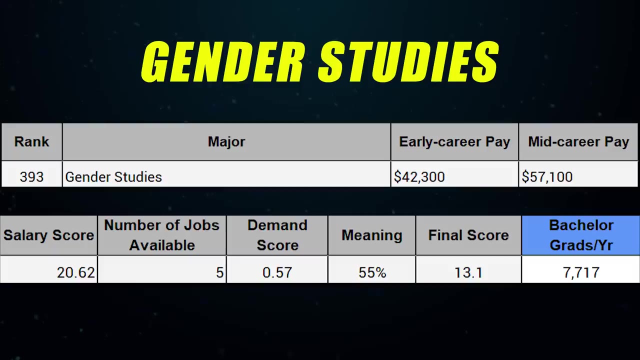 pretty interesting. goes into B tier Anthropology at the bachelor's level. this one has to go into F tier Management information systems- great degree. it goes into S tier Gender studies. goes into F tier Criminology. goes into D tier Music. is going to go into F- Computer. 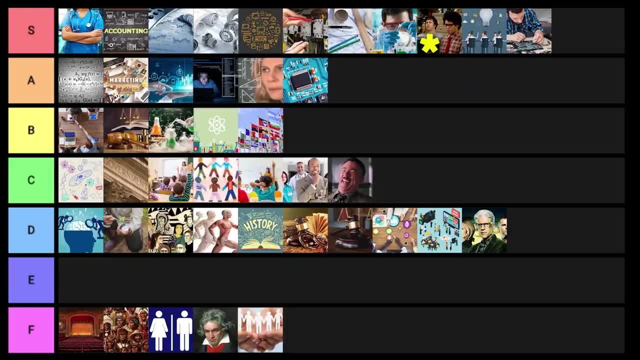 engineering is S Human services goes into F- Biomedical engineering- that's going to go into B tier. And then there's a lot of different things that can be done here. But if you're going to go into A tier, that one is going to make it into low S tier status. Bioengineering is: 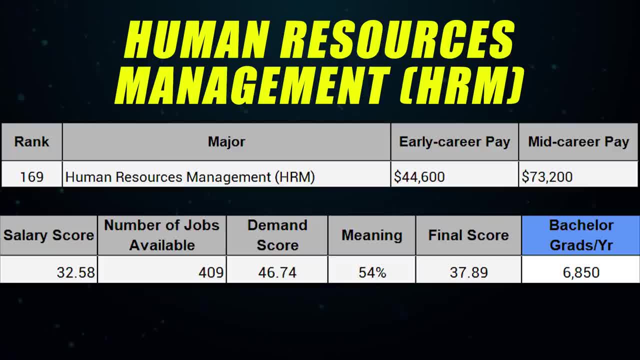 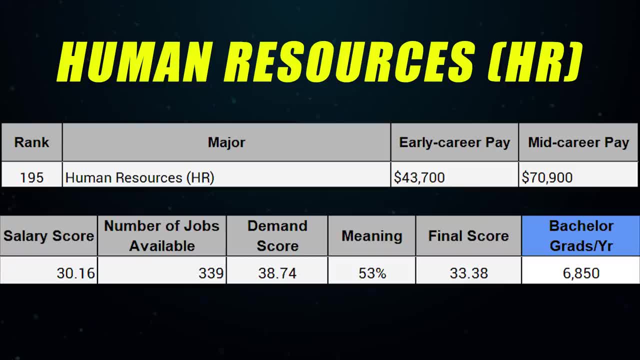 going to be high A tier Physics. I'm going to go ahead and put this one into low S tier. Human resource management: this one is interesting. I'm going to put it into C tier. Same with human resources. Environmental science is going to go into C tier- low C tier, I'd. 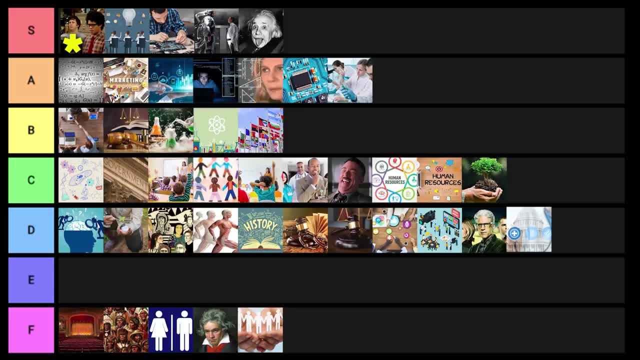 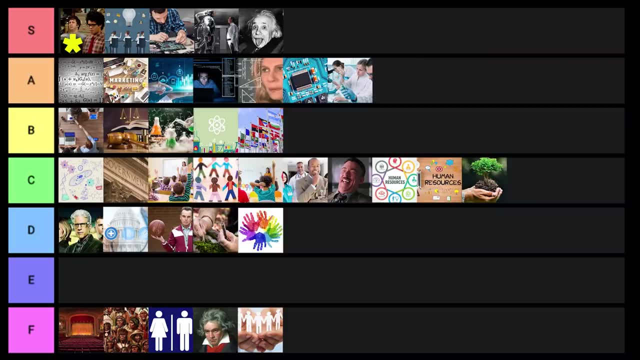 say, Public health goes into D. tier. Physical education teaching: this one's going to go into D. tier Environmental studies: This is going to go into this. one also goes into D. Special education's going into D as well. Spanish language: this one's gonna go into D. 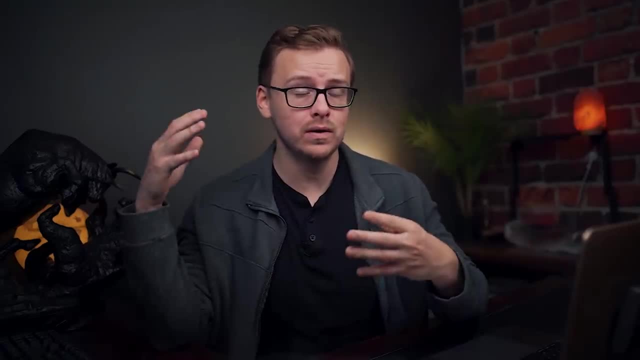 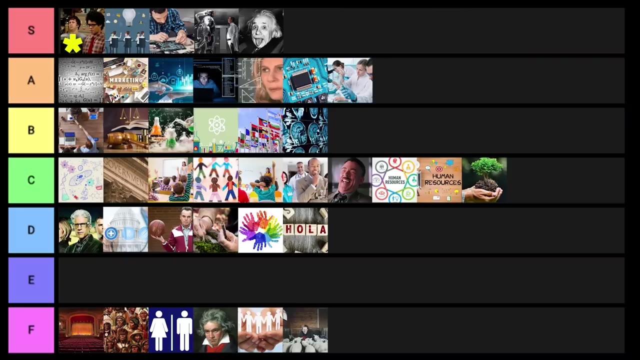 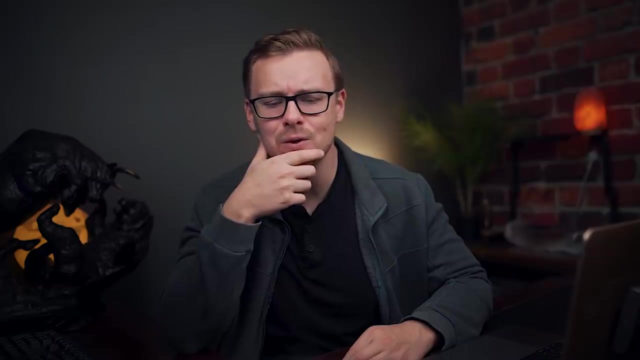 Animal science at the bachelor's level, if you're not also planning on going to veterinary school. this one goes into F tier. Neuroscience is gonna go into B tier. International business is going into A. Philosophy goes into C tier. Geology- I would say high B tier or low A tier. 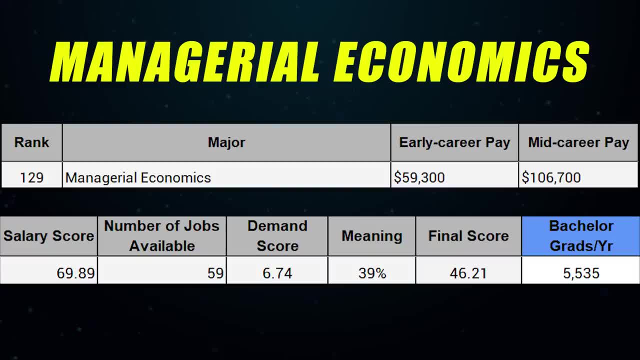 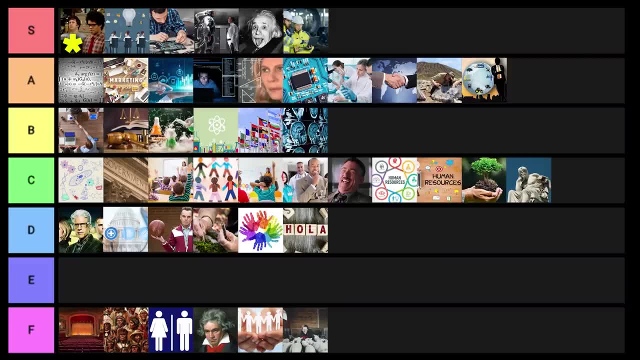 Ooh, this one's kind of tough. I'll give it low. A tier: Managerial economics, another one I would probably put into A tier: Industrial engineering. S tier, Interdisciplinary studies. F tier, Supply chain management. I'll go ahead and put it into A. 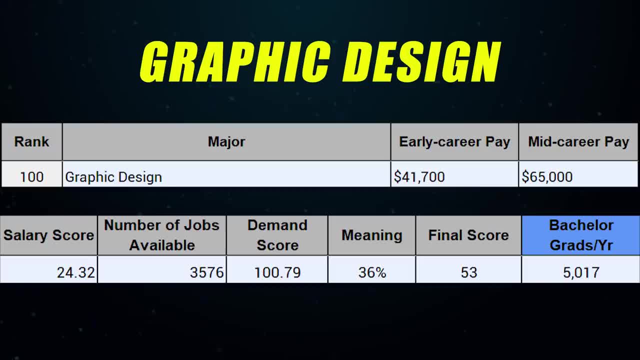 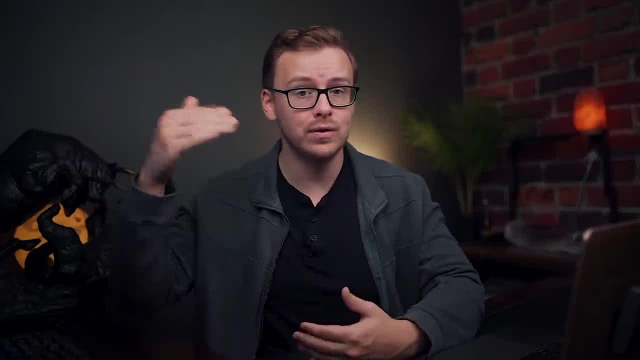 Architecture. I'll go ahead and put this one into B tier- Graphic design, C tier, Communication sciences and disorders at the bachelor's level. not planning on going and becoming a speech language pathologist, for instance, Definitely is gonna go into F tier. 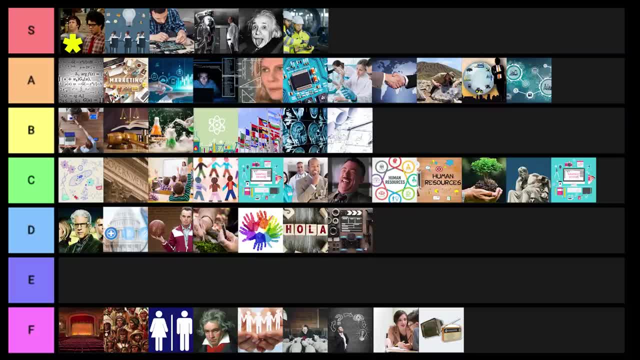 Radio and television- F tier. Video production- D tier. Advertising- this one goes into A tier. Multimedia: D tier. Aerospace engineering is gonna go into S tier. Aeronautical engineering goes into A tier. Athletic training- F tier. 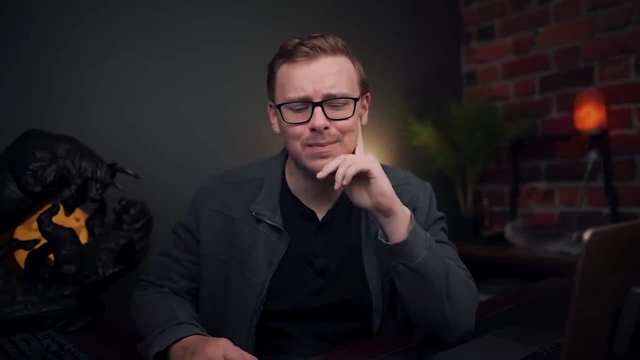 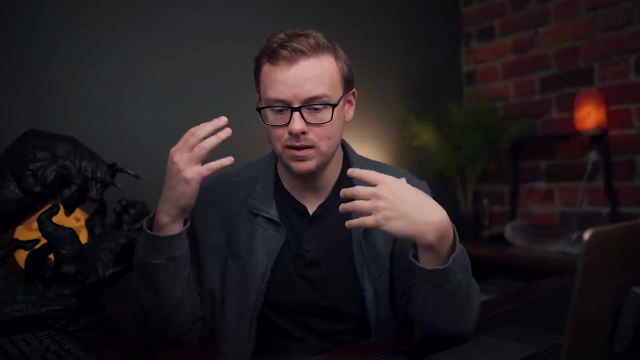 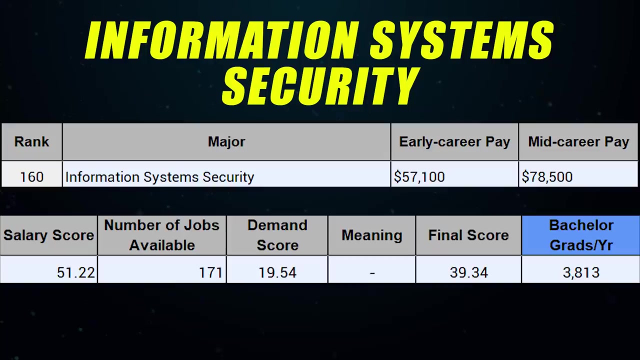 Organizational leadership, I'd say probably D tier- Exercise physiology again at the bachelor's level. you're not planning on becoming some type of physical therapist or something along those lines? I would put this one into D tier, Information systems security. I'll go ahead. 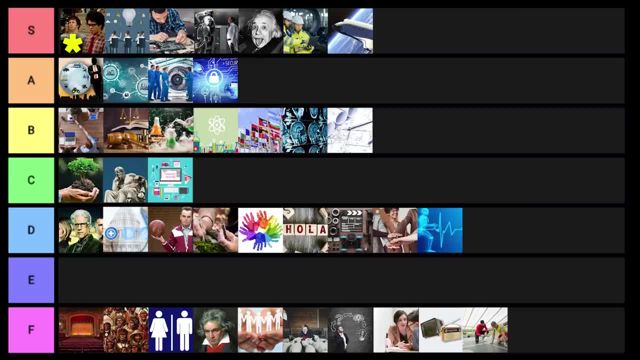 and put this one into A tier- Geography. I'll put it into C tier- Education: C tier- Cinema studies. F tier- Film studies. F tier- Management science. B tier- Family and consumer science. F tier- And last one on the list, nutrition science.